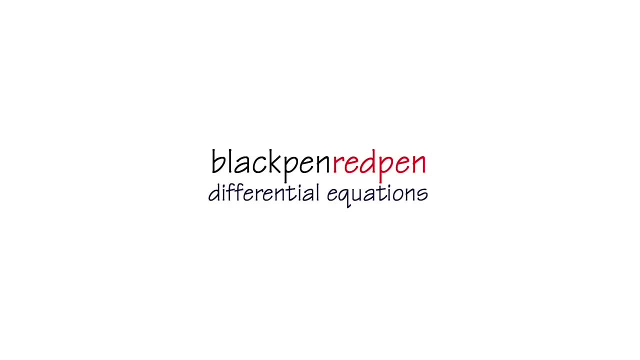 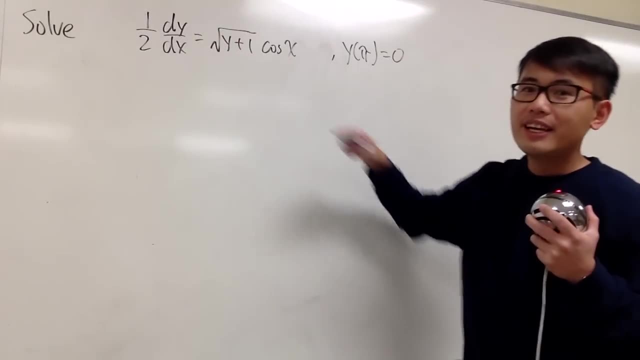 Black pen, red pen. yeah, Let's solve this differential equation. We have 1 half dy: dx is equal to square root of y plus 1 times cosine x. And we also know y of pi is equal to 0. So be sure to solve for that constant. 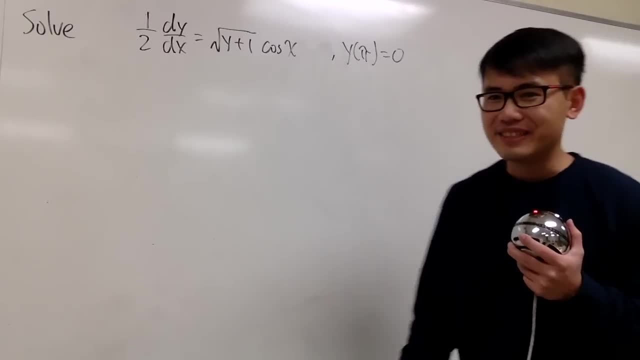 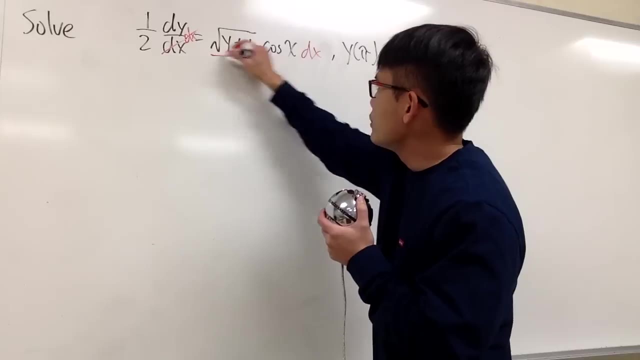 And I will have to talk about when we should solve for that constant in this video. Okay, let's go ahead and do our usual business. Let's go ahead and multiply dx on both sides, And I would also like to divide both sides by square root of y plus 1.. 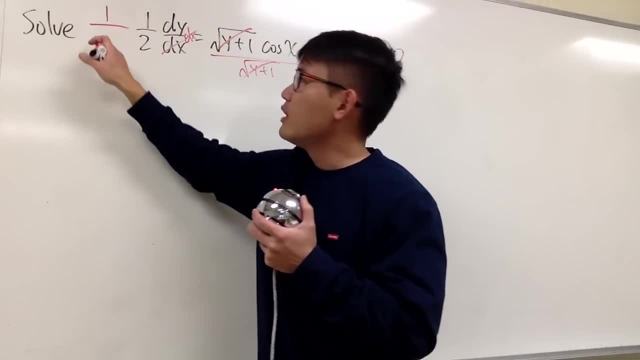 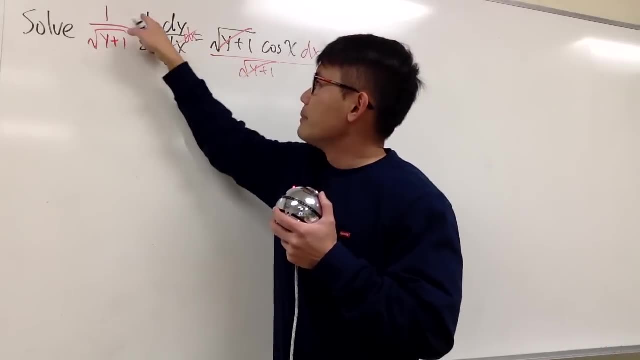 And on the left-hand side. let me just put this down as 1 over square root of y plus 1, like this: Okay, to clean things up, on the left-hand side, 1 times 1 is just 1. And we'll write this down as 1 over. 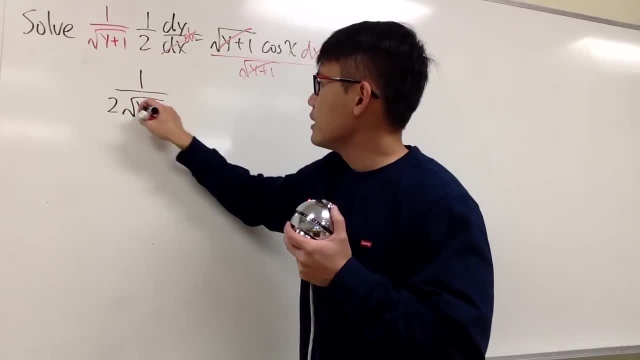 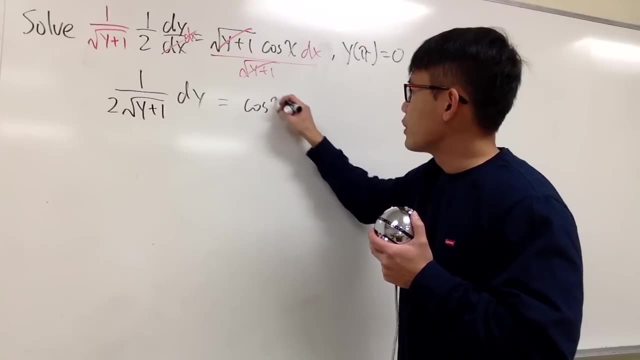 Put a 2 in the front, 1 over 2 square root of y plus 1.. And we have the dy here And that's equal to on the right-hand side, which is of cosine x, dx, And we're ready to integrate, integrate right. 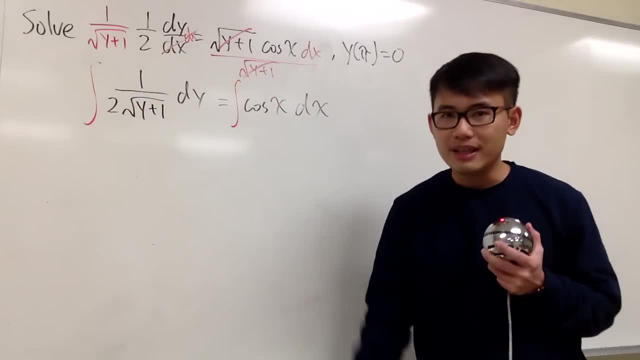 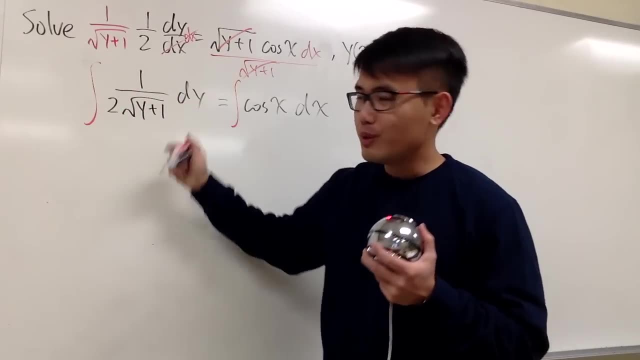 Because all the y's and all the x's, they are in the right place. What's the integral of 1 over 2? square root of y plus 1? This right here is just going to be square root of y plus 1.. 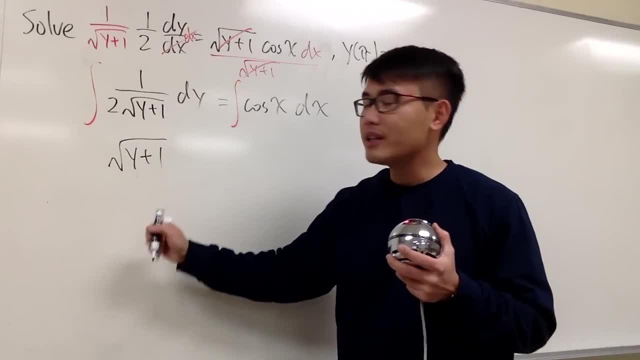 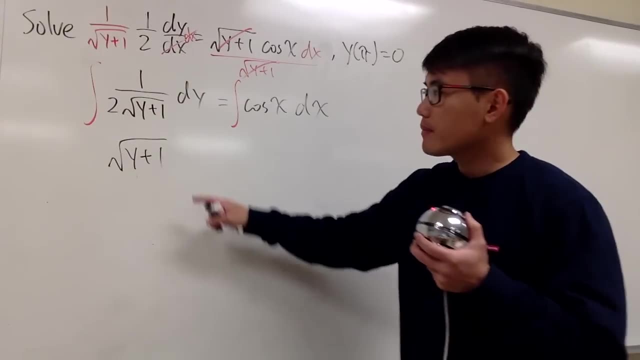 Because a few ways you can do it. Of course you can use u substitution that u is equal to y plus 1.. Go to the usual step, right? But I will suggest you guys to do it this way: Look at the inside and you know that the derivative of y plus 1 is just 1.. 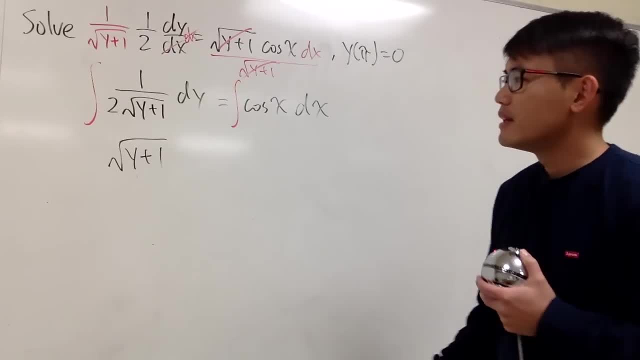 So you don't have to do it this way, You don't have to divide or multiply by any constants And you know the general form: 1 over 2, square root of something is going to give you square root of something, okay. 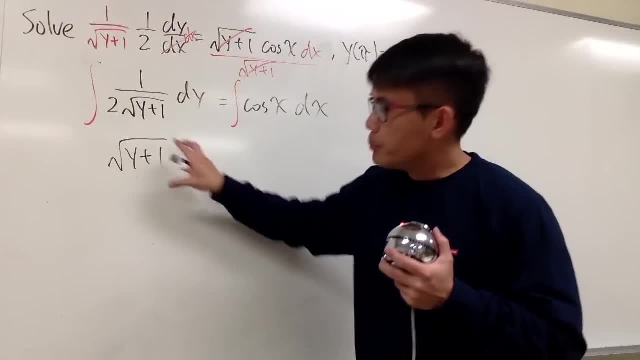 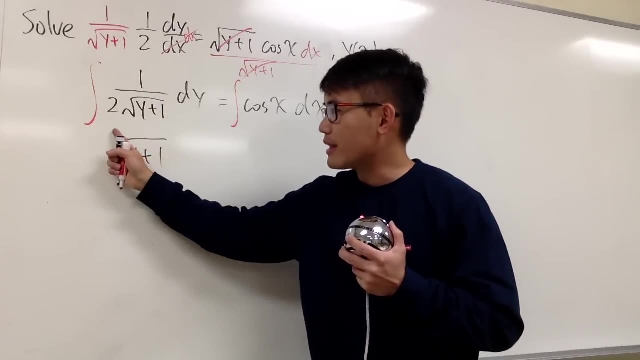 And the best way to do it is you integrate this in your head, Put down the answer just like this And differentiate the answer and see if you can get back to this. Okay, let's go ahead and do that. Differentiate square root of y plus 1.. 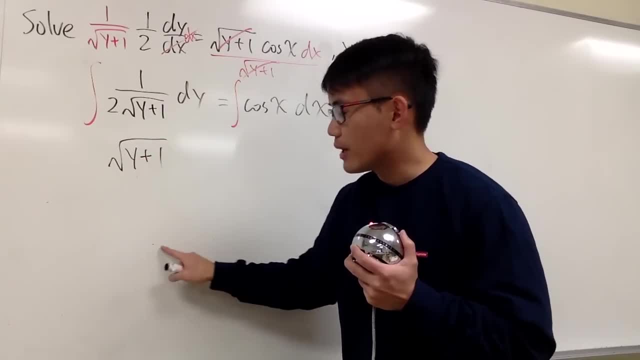 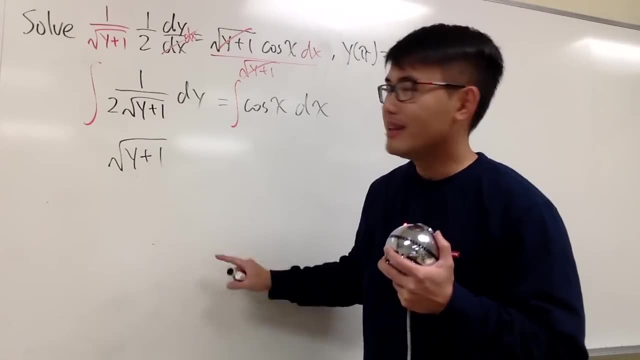 We first get 1 over 2, square root of the inside right, y plus 1. And you multiply by The derivative inside. by the chain rule, The derivative of y plus 1 is just 1. And you get back to the original. 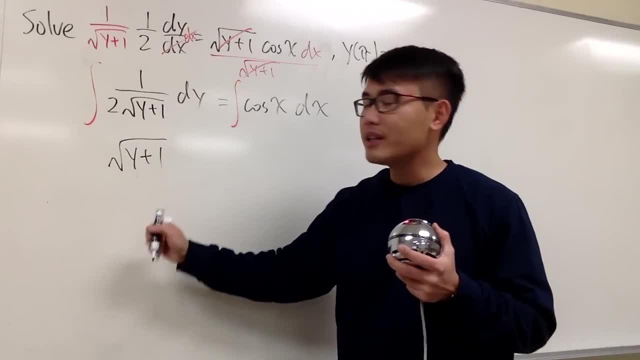 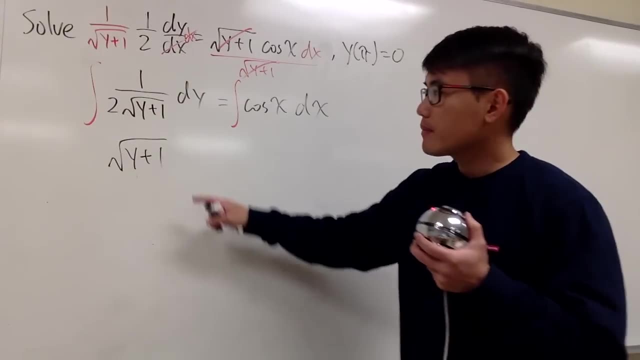 Because a few ways you can do it. Of course you can use u substitution that u is equal to y plus 1.. Go to the usual step, right? But I will suggest you guys to do it this way: Look at the inside and you know that the derivative of y plus 1 is just 1.. 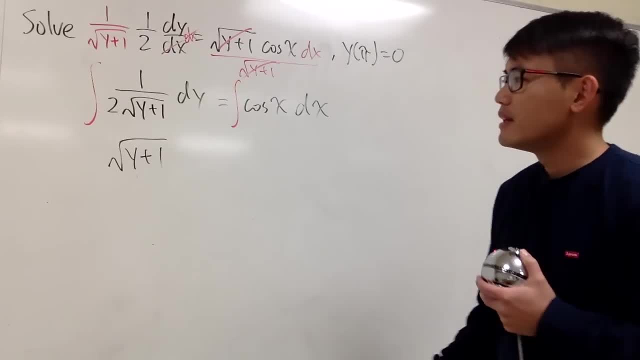 So you don't have to do it this way, You don't have to divide or multiply by any constants And you know the general form: 1 over 2, square root of something is going to give you square root of something, okay. 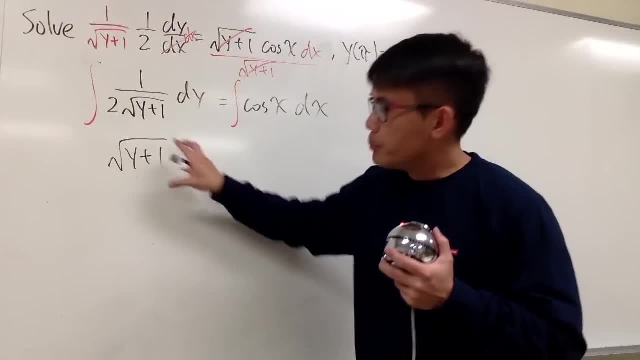 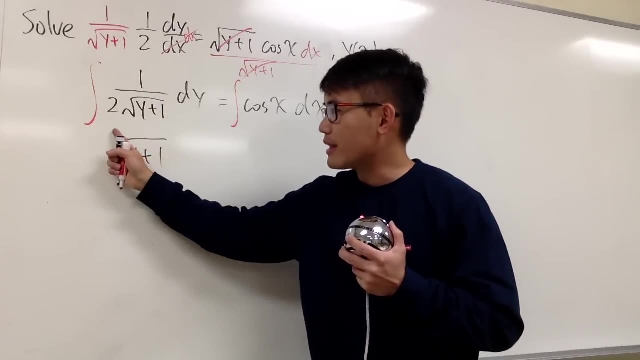 And the best way to do it is you integrate this in your head, Put down the answer just like this And differentiate the answer and see if you can get back to this. Okay, let's go ahead and do that. Differentiate square root of y plus 1.. 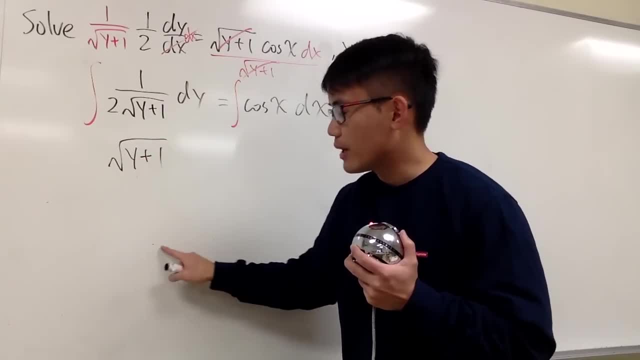 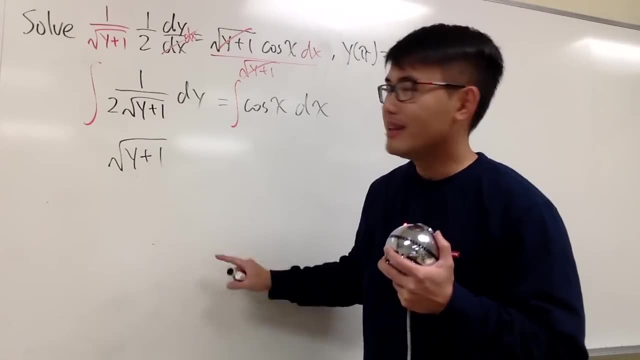 We first get 1 over 2, square root of the inside right, y plus 1. And you multiply by The derivative inside. by the chain rule, The derivative of y plus 1 is just 1. And you get back to the original. 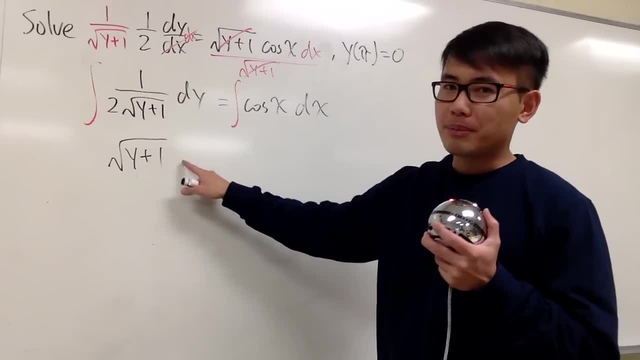 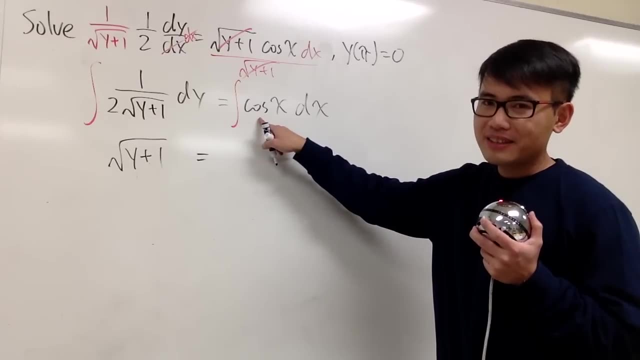 Okay, so right here. this is it. You don't have to worry about the plus constant on the left-hand side. We can just write this down: This is equal to, And the integral of cosine x is positive sine x. Okay. 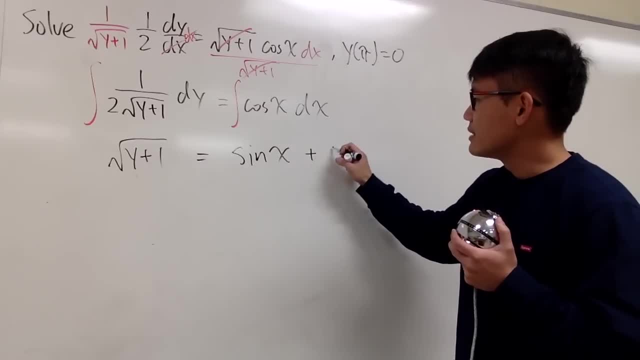 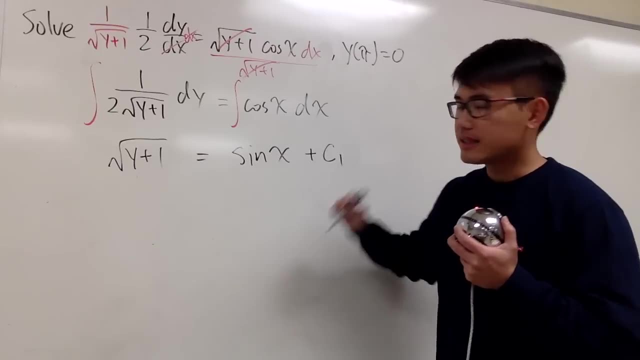 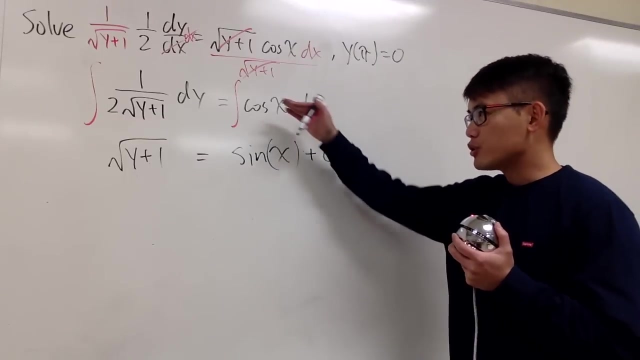 Let's write this down. And let me just write down plus c1 right here And let me emphasize that the plus c1 is after the sine x. So let me use the parentheses right here to close it, to emphasize that. Okay, now we are pretty much done with the integration part, with the solving part for the differential equation. 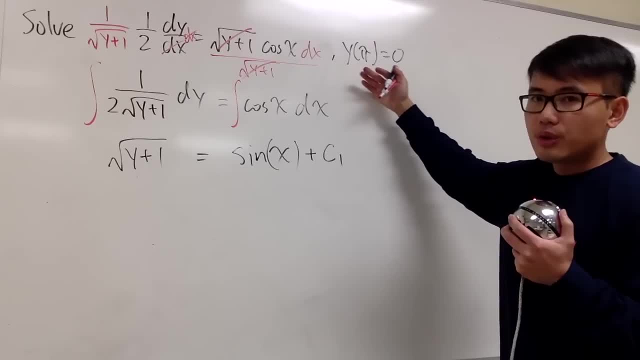 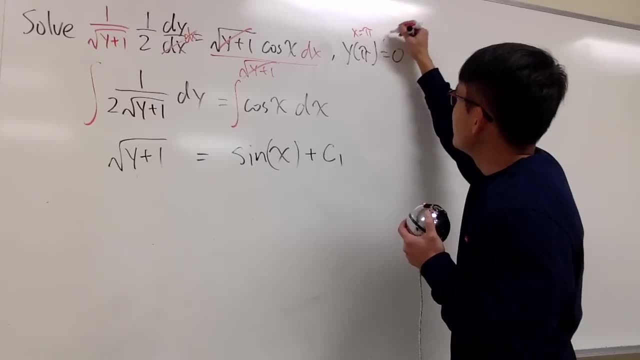 And because we're given this initial value, in this case I would like to plug in: x is pi And that will give us y will be 0.. I would like to plug in these values right here to solve for c. It's because 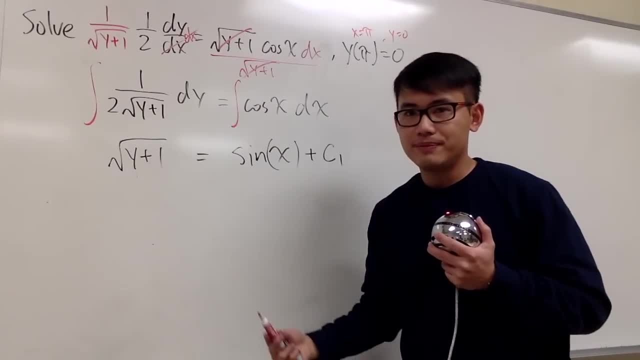 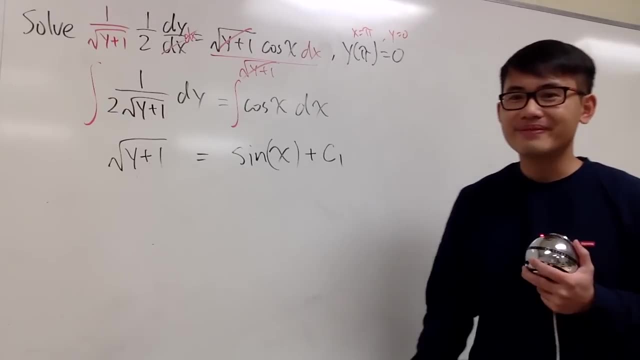 It's because if you isolate the y first and then want to solve for c later on, you wouldn't know if c should be positive or negative. Let me just do it the way I want to show you guys right here. I would like to solve for c now. 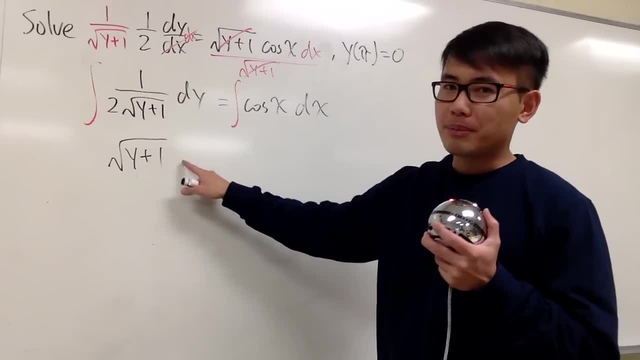 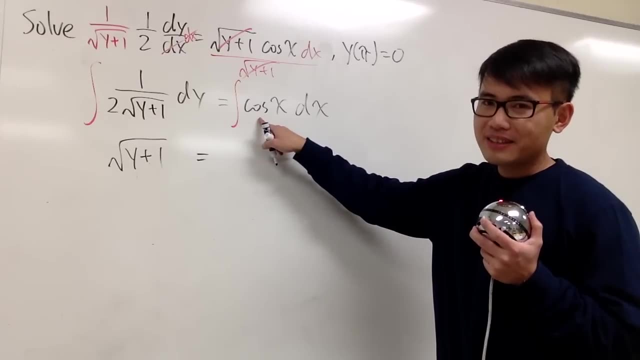 Okay, so right here. this is it. You don't have to worry about the plus constant on the left-hand side. We can just write this down: This is equal to, And the integral of cosine x is positive sine x. okay. 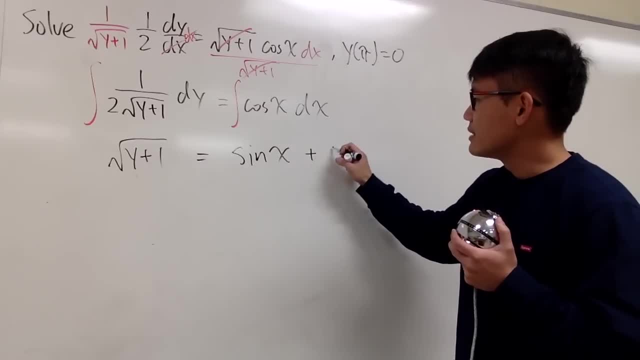 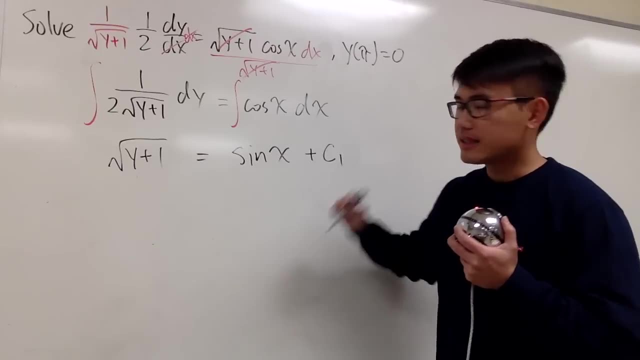 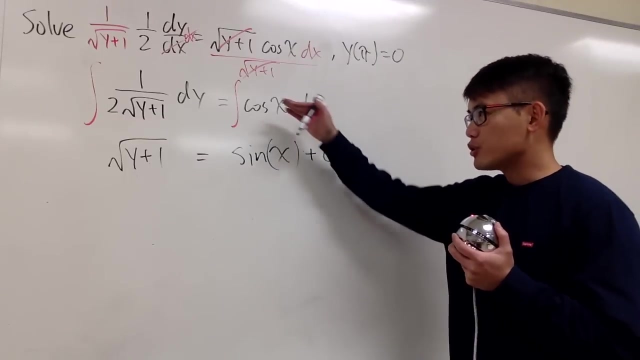 Let's write this down. And let me just write down plus c1 right here And let me emphasize that the plus c1 is after the sine x. So let me use the parentheses right here to close it, to emphasize that. Okay, now we are pretty much done with the integration part, with the solving part for the differential equation. 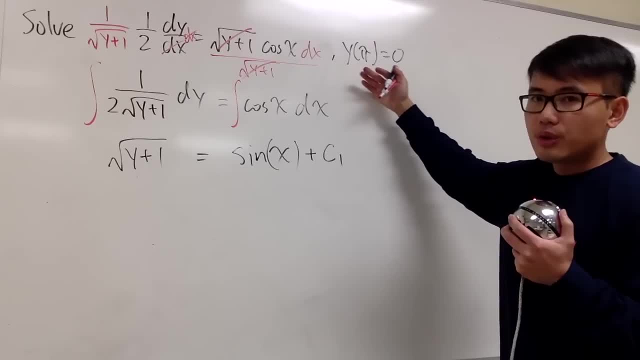 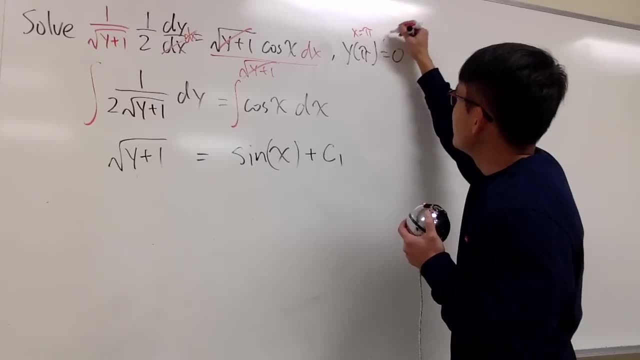 And because we're given this initial value, in this case I would like to plug in: x is pi And that will give us y will be 0.. I would like to plug in these values right here to solve for c. It's because 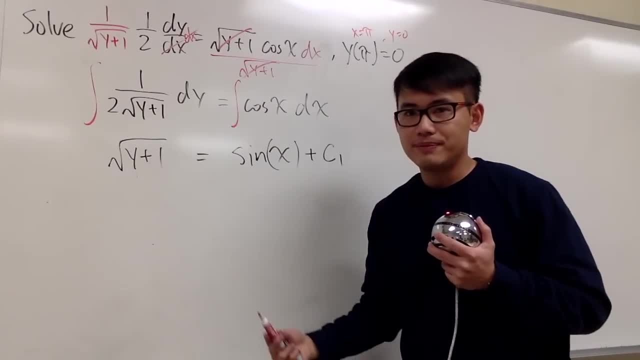 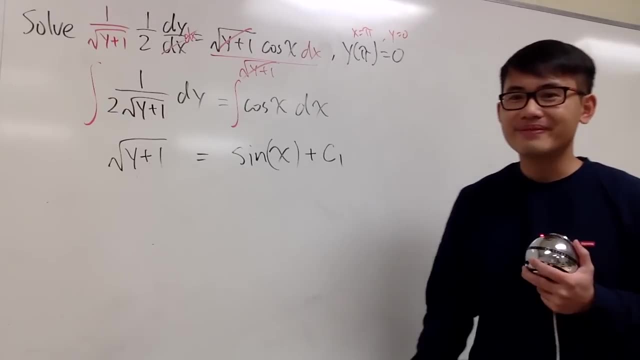 It's because if you isolate the y first and then you want to solve for c later on, you wouldn't know if c should be positive or negative. Let me just do it the way I want to show you guys right here. I would like to solve for c now. 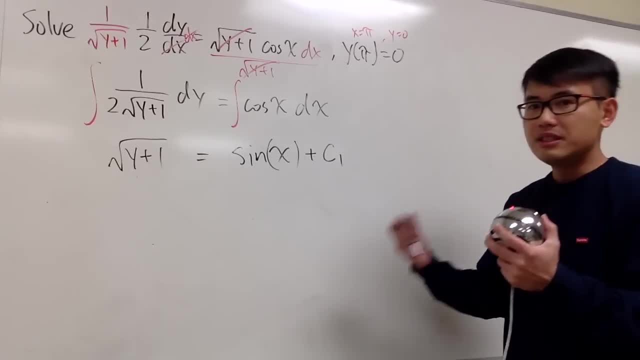 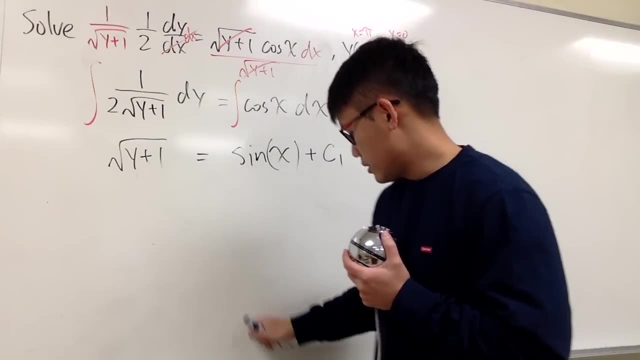 And I will show you guys what I mean by. we wouldn't know if c is negative or not later on. Okay, plug in 0 into this y. here We have 0. here Let me get the right color, 0 and then plus 1.. 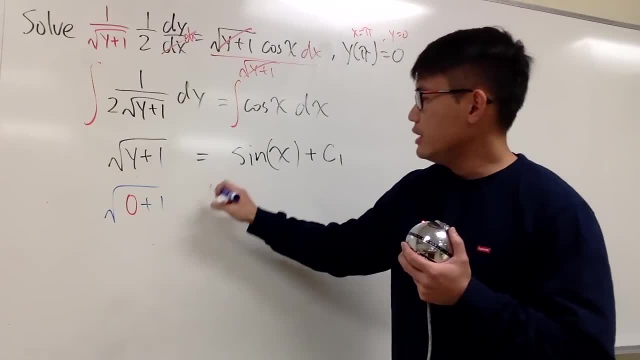 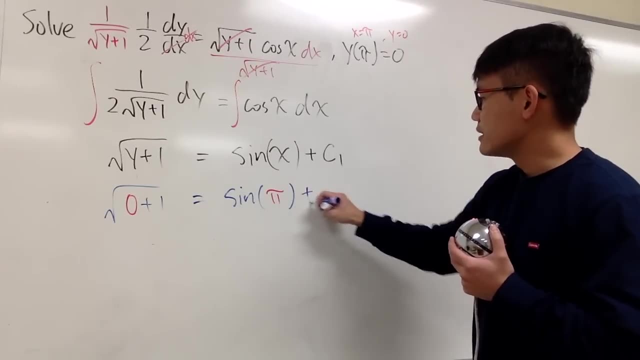 And then that's inside the square root And this is equal to. We have the sign x is pi And we close that, And then we add the c. Well, technically we're just using the c right here, So you don't need to label it c1.. 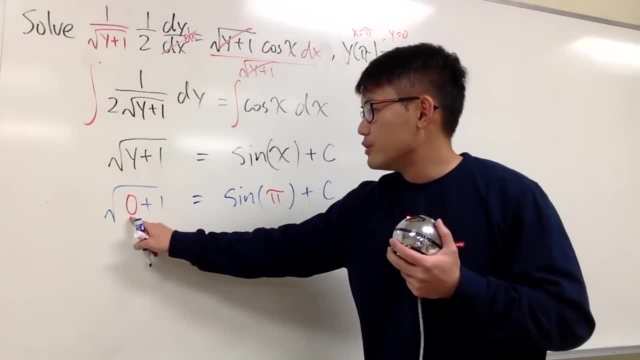 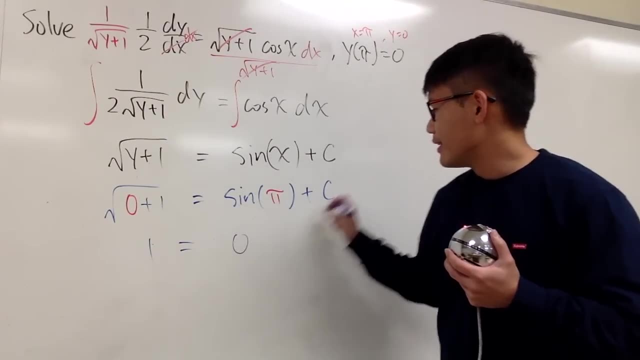 Just the c. Okay, 0 plus 1 is 1.. Square root of 1 is just 1.. This is equal to sine of pi is 0. And then plus c. So of course you see, c is equal to 1.. 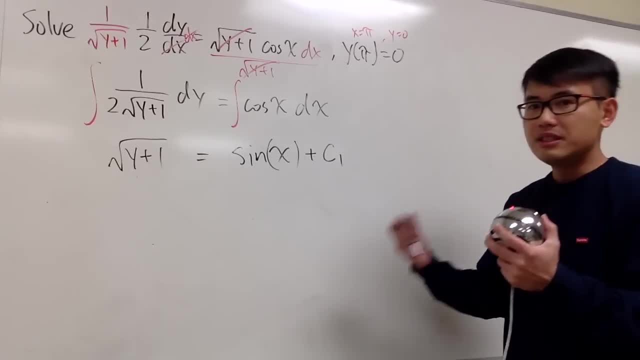 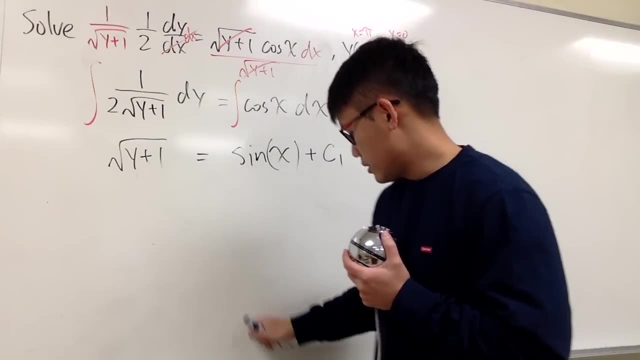 And I will show you guys what I mean by. we wouldn't know if c is negative or not later on. Okay, plug in 0 into this y. here We have 0. here Let me get the right color, 0 and then plus 1.. 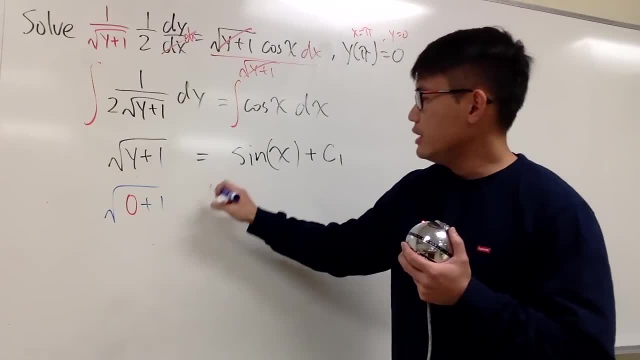 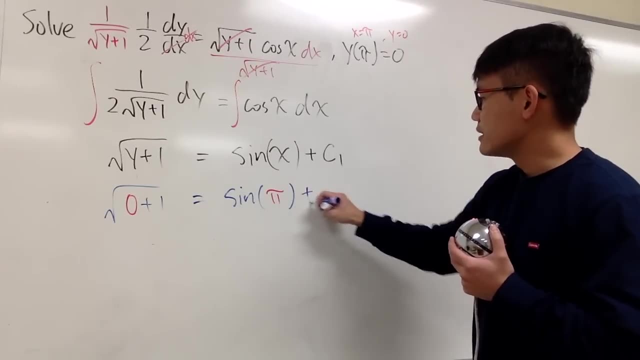 And then that's inside the square root And this is equal to. We have the sign x is pi And we close that, And then we add the c. Well, technically we're just using the c right here, So you don't need to label it c1.. 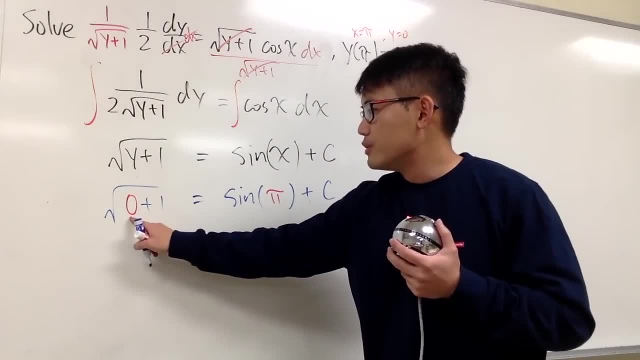 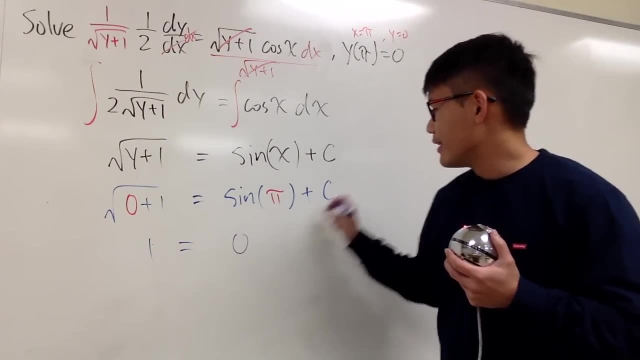 Just the c. Okay, 0 plus 1 is 1.. Square root of 1 is just 1.. This is equal to sine of pi is 0. And then plus c. So of course you see, c is equal to 1.. 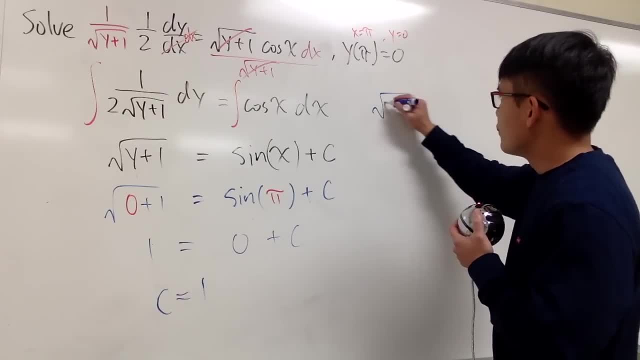 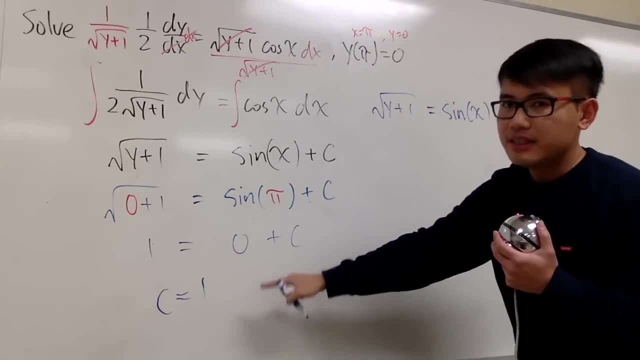 And you're pretty much done. So here you have square root of y plus 1 is equal to sine of x. See, in this case, as you can see, it's positive 1, right, So we add the 1 after that. 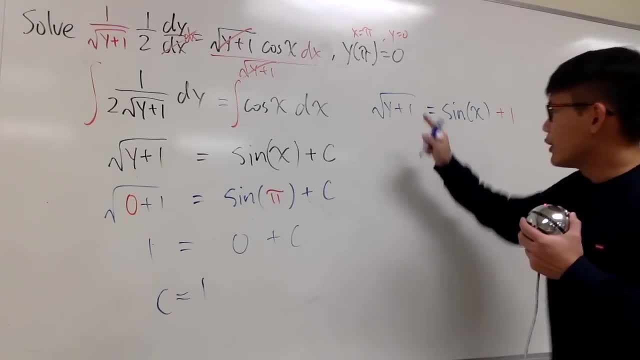 At the end, this is not bad to do, So we'll do it. We would like to isolate y, So let's go ahead, square both sides. They cancel And we will have. y plus 1 is equal to sine of x plus 1 inside of this big parentheses. 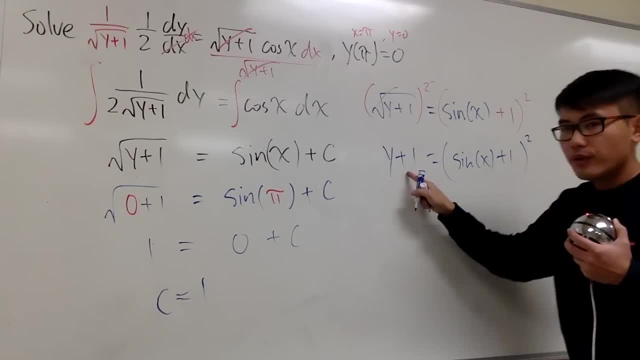 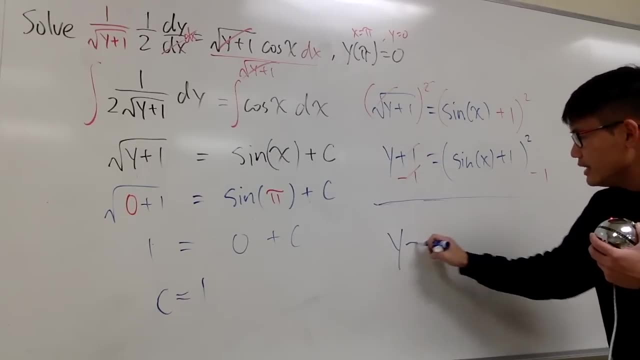 And square that. And of course we have to just subtract 1 on both sides And we see that y is equal to sine of x, and then plus 1.. And then square that And then minus 1.. Here is the answer. 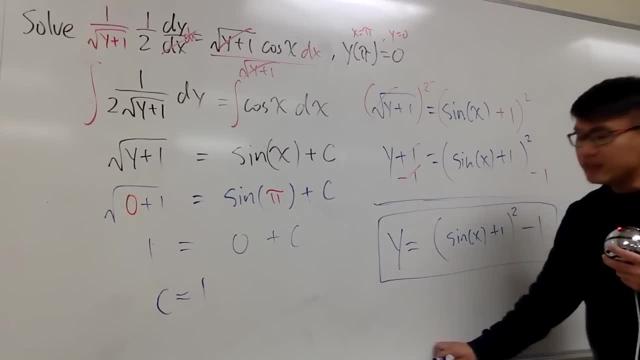 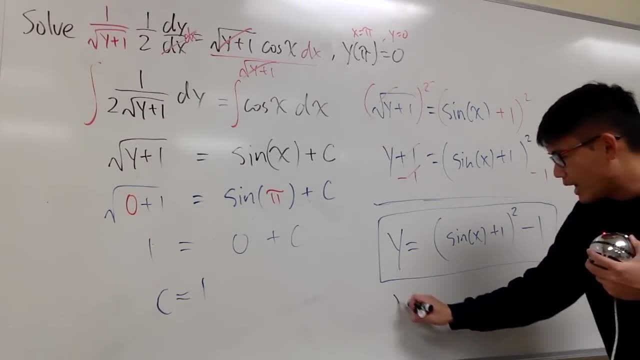 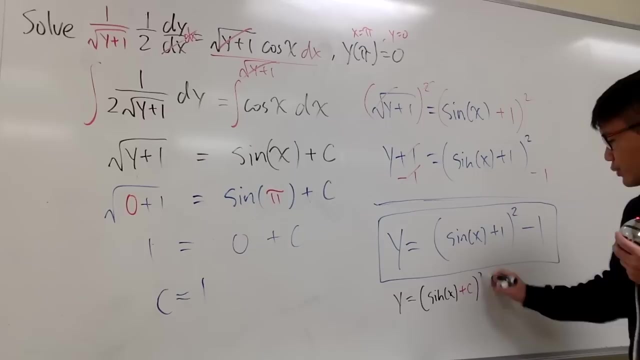 Okay, All right. So real quick. imagine if you isolate the y first, And this is where the c was right. So if you isolate the y first, you will have: y is equal to sine of x plus the c, which we don't know what it is. 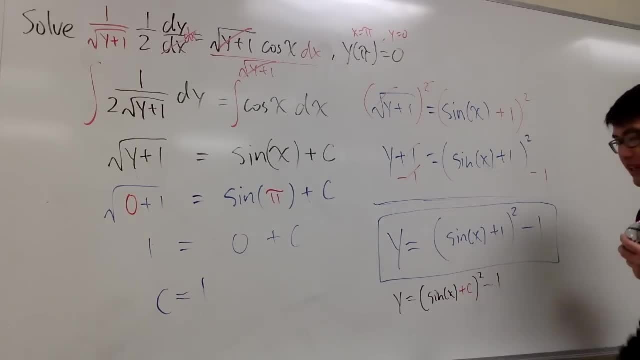 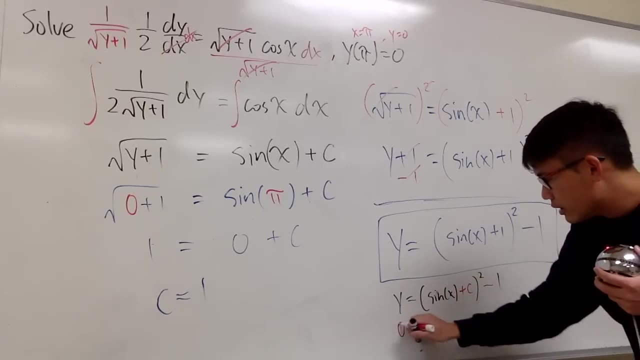 And you square that: This is my sine of x, And then minus 1 after that. Imagine if you get this first And you plug in these values 0 into y, And this is going to give you. This is sine of pi for the x. 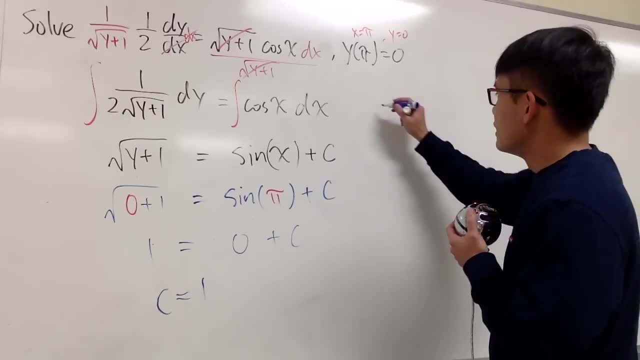 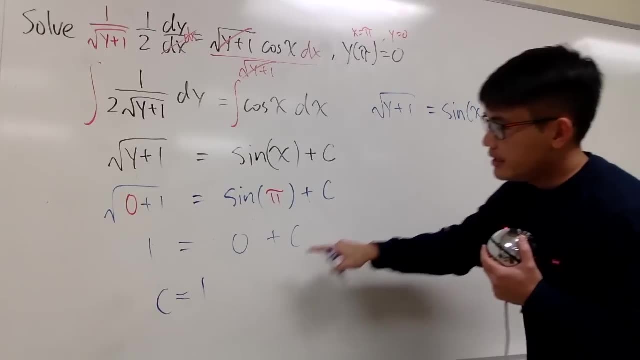 And you're pretty much done. So here you have: square root of y plus 1 is equal to sine of x. See, in this case, as you can see, it's positive 1, right, So we add a 1 after that. 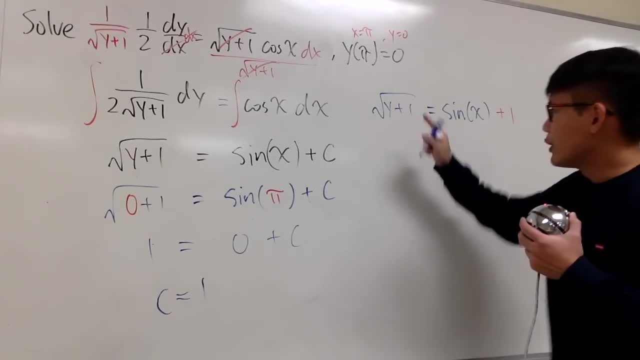 At the end, this is not bad to do, So we'll do it. We would like to isolate y, So let's go ahead, square both sides, They cancel And we will have. y plus 1 is equal to sine of x. 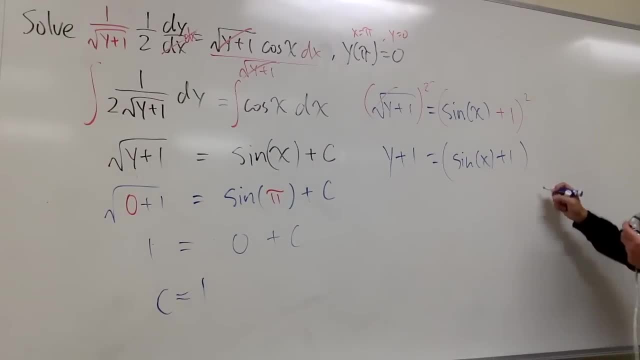 Plus 1, inside of this big parentheses And square that. And of course we have to just subtract 1 on both sides And we see that y is equal to sine of x, And then plus 1.. And then square that. 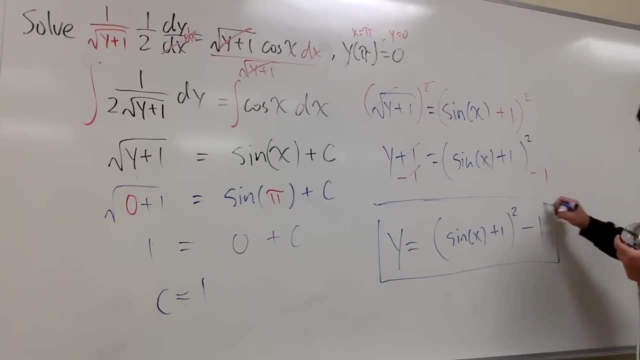 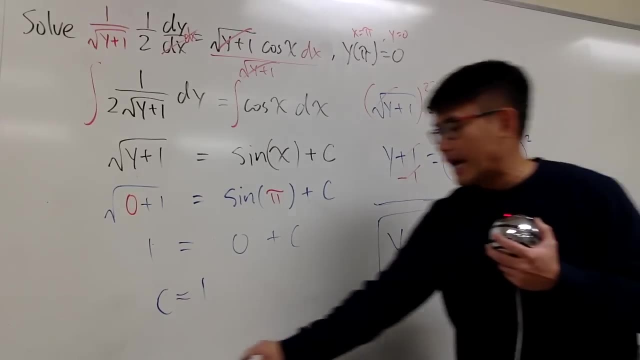 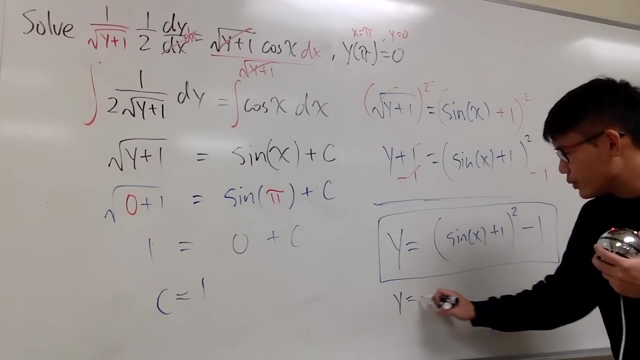 And then minus 1.. Here is the answer. Okay, All right. So real quick. You isolate the y first, And this is where the c was right. So if you isolate the y first, you will have: y is equal to sine of x plus the c. 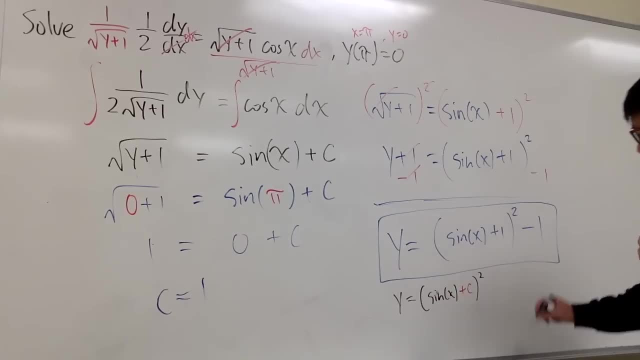 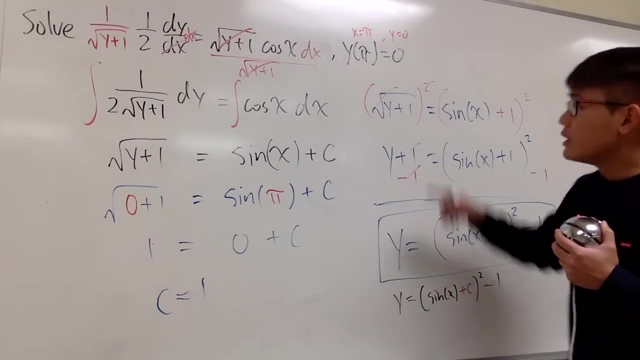 which we don't know what it is, And you square that- This is my sine- of x And then minus 1 after that. Imagine if you get this first And you plug in these values 0 into y And this is going to give you. 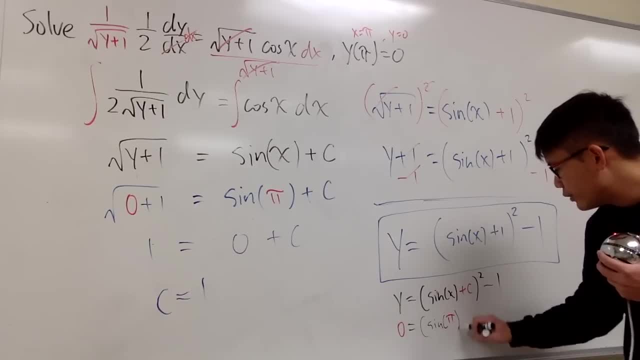 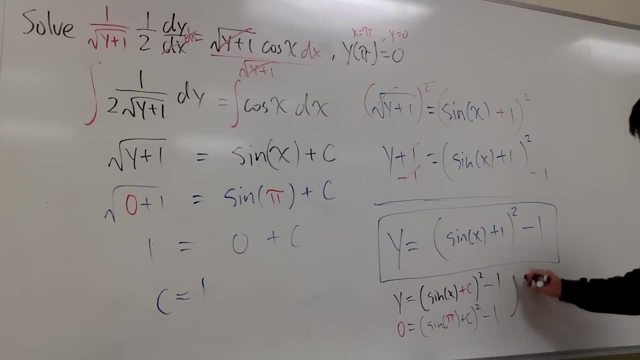 This is sine of pi for the x, And you add a c after that And you square that And then minus 1.. You see This is 0.. And sine of pi is 0 plus c, So it's just c inside. 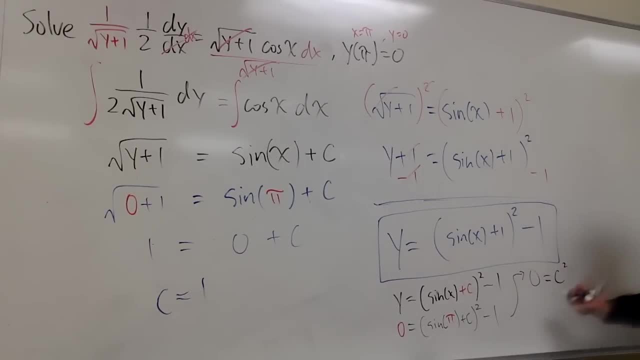 We have c squared, This is equal to c squared And we have the minus 1.. You can add one on both sides. You have c squared, It's equal to 1.. You see, If you isolate the y first earlier, 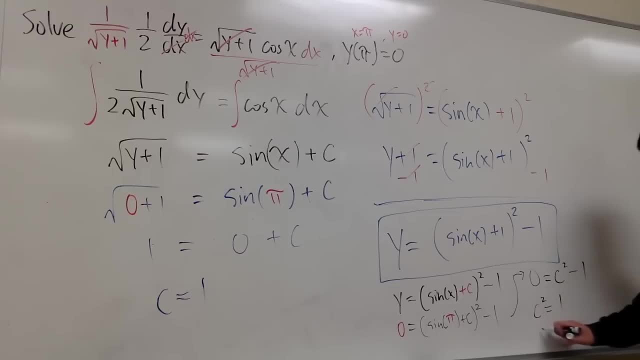 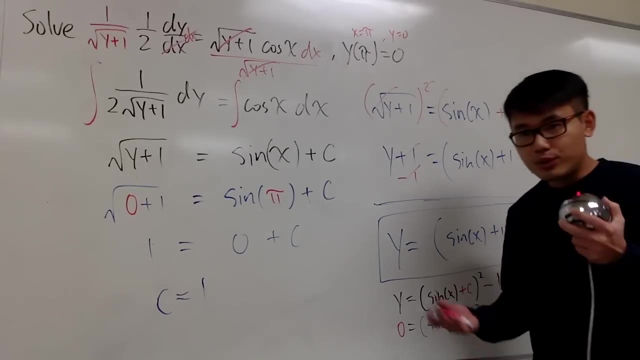 you end up with c squared, It's equal to 1.. And are you going to say c is 1? Or c is equal to negative 1?? Well, to decide, you actually have to look back to this part of the equation.